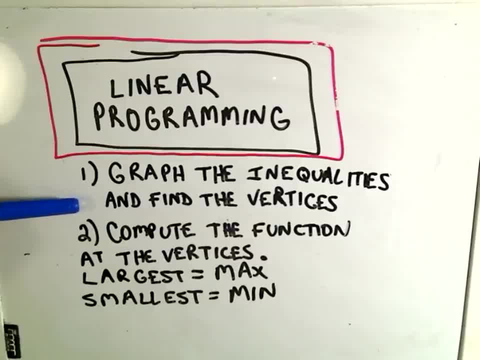 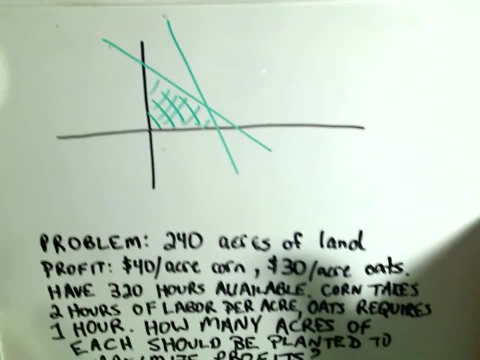 Find the vertices, which are basically just the corners of the region. You'll basically plug those corner points into the function. whatever the largest value is at your maximum, the smallest is your minimum. So here's basically just a little example of what's going to happen. 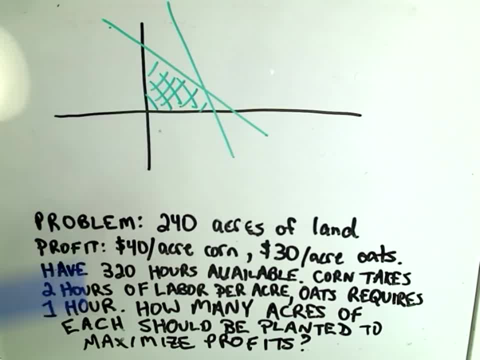 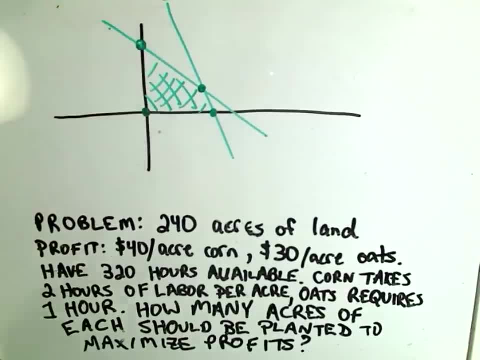 You'll graph your region, your inequalities. You'll find some little region- here It's in the green Again. you'll basically just find the vertices, the corners, plug those in and determine which one's a max and which one's a minimum. 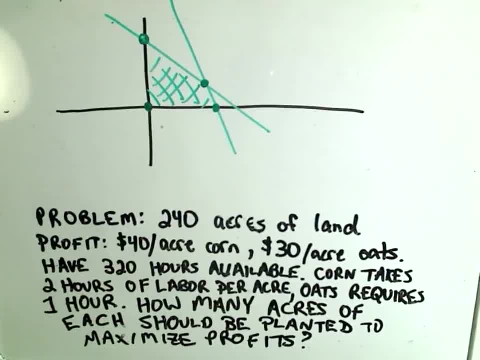 Okay, so here's our actual problem that we'll do here. So suppose you have 240 acres of land And you're going to, You can make $40 per acre for the corn, $30 per acre of oats that you plant. 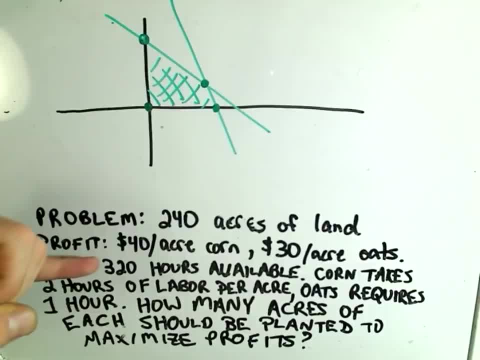 But it takes an hour to harvest the stuff. So suppose you have 320 hours available and it takes two hours of labor per acre, for the corn And oats only take one hour of labor. So how many acres of each should be planted to maximize profits? 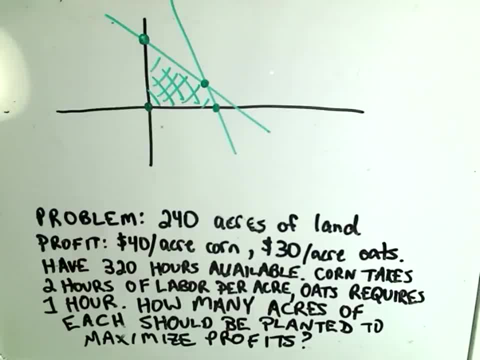 Okay, so, intuitively, you know, you'd probably like to plant. Okay, so, intuitively, you know, you'd probably like to plant a lot of Well, I don't know, It's a trade-off, right. 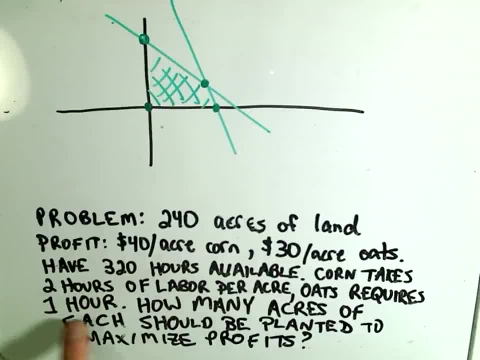 If you plant corn you get more money. But you know you can do two hours. You can harvest two acres of oats for every one acre of corn, But you actually double your money then. But then of course you're taking up extra space. 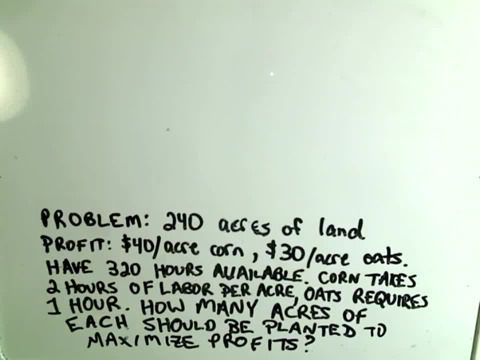 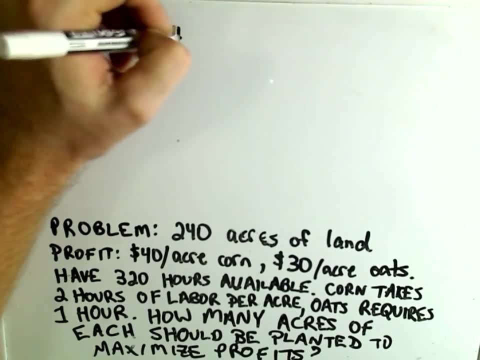 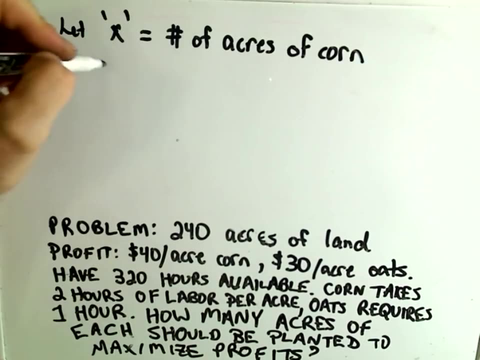 So Alright, so there's some issues here, So let's see if we can't figure it out. So I'm going to let x equal the number of acres, equal the number of acres of corn that we'll plant, And then the same thing. 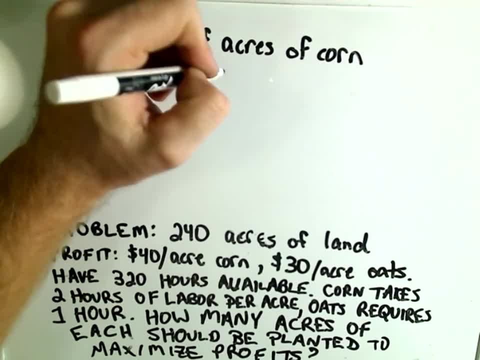 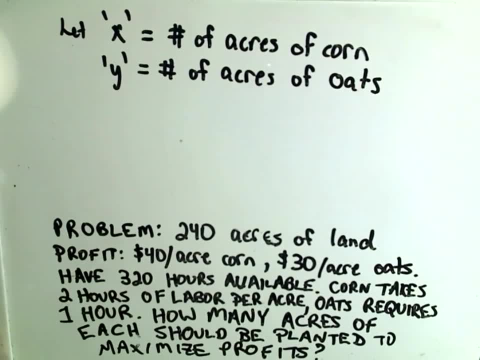 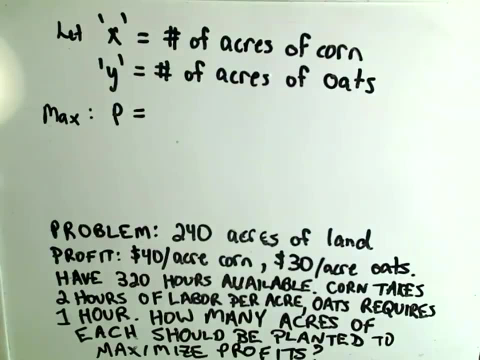 We'll let y equal the number of acres of oats that we plant. Okay, the thing that we're trying to maximize here, in this case, we want to maximize our profit. Well, what would our profit be? Well, for every acre of corn you get. 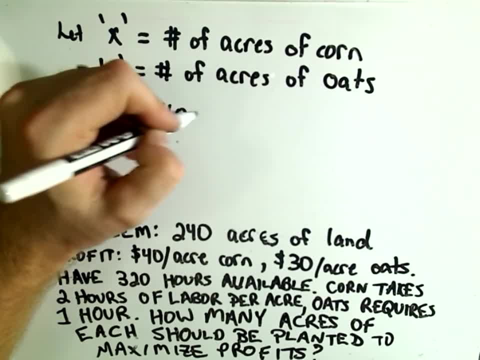 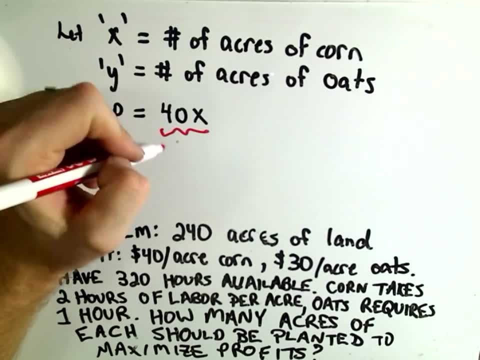 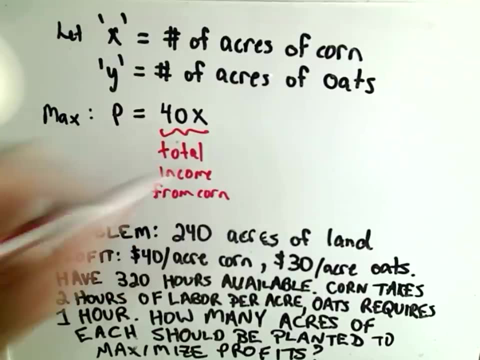 basically $40.. So we'll take 40 and multiply it by the number of acres of corn And this will represent the total income, the total income from the corn. And then we'll add to that 30 times y And that'll represent simply the total income. 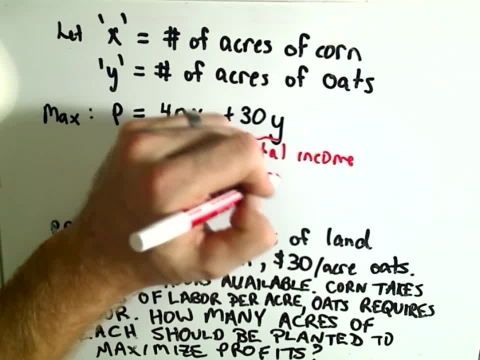 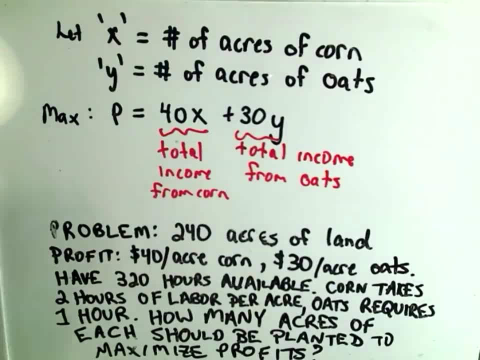 that'll be the total income from the oats if we plant y acres. Okay, so we also have some other constraints here. We only have 240 acres of land. Well, so that's where we're going to get some of our constraints here. 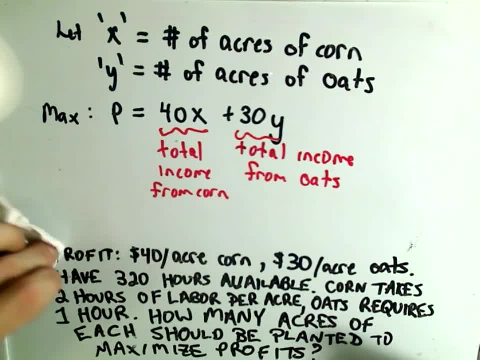 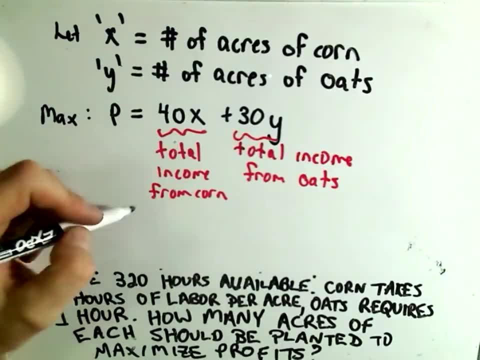 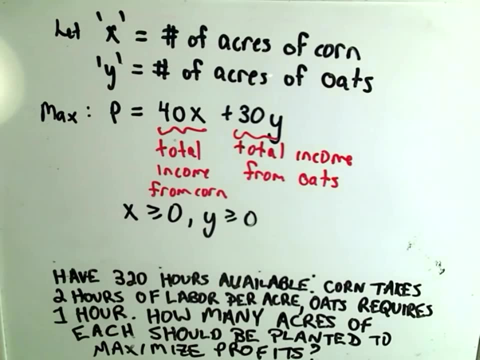 Okay, so we've taken care of the profit. Okay, so we only have 240 acres of land. Well, certainly as well, notice, we'll have the inequalities. x has to be greater than or equal to 0.. y has to be greater than or equal to 0. 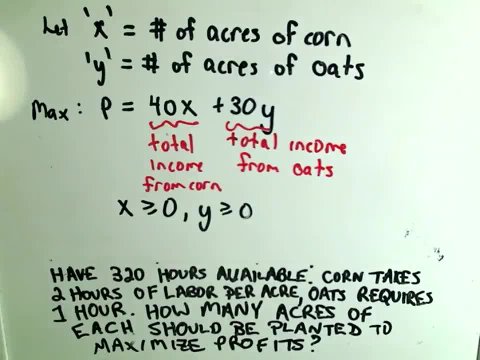 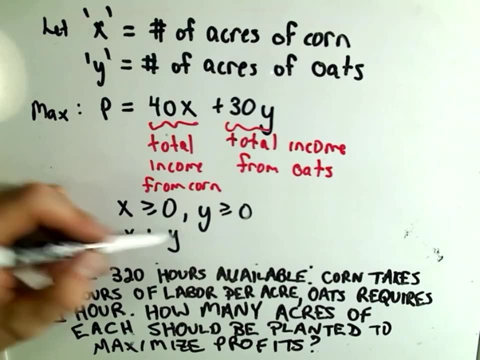 because you can't. you know, you can either plant 0 or some positive number of acres. Notice also: one of our inequalities is that x plus y- Okay. so we're planting x acres of corn, y acres of oats. This represents the total number of acres. 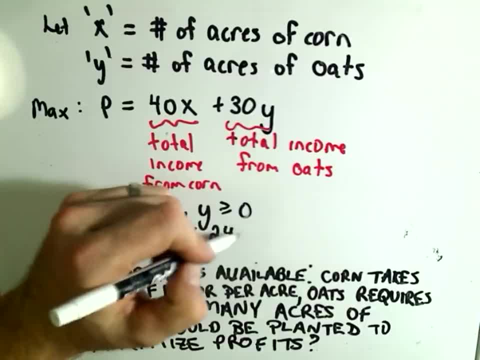 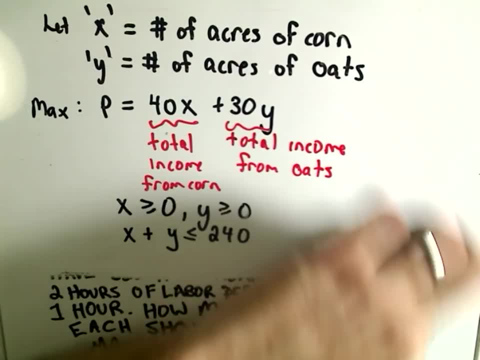 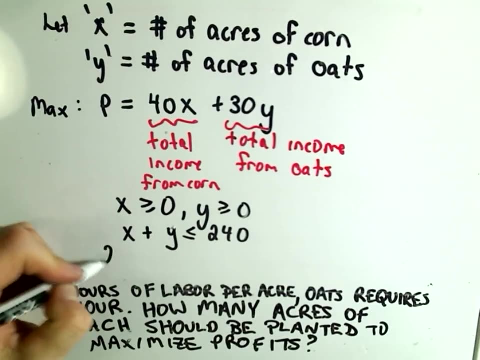 And we know that the total number of acres has to be under less than or equal to 240.. Likewise, we only have 320 hours available- man hours- to accomplish our task. So it takes 2 hours per acre of corn plus 1 hour per acre of oats. 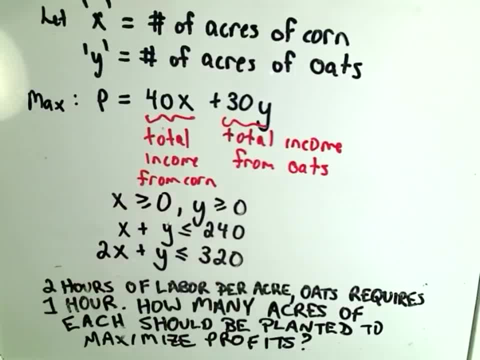 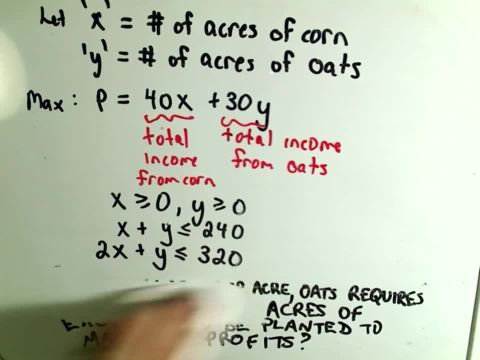 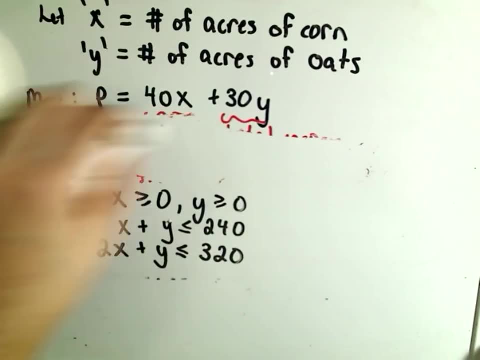 And we know that that has to be less than or equal to 320.. Okay, because that's how much time we have available. So these are going to be our systems of inequalities here that we're going to have to graph here. So let me erase this part. 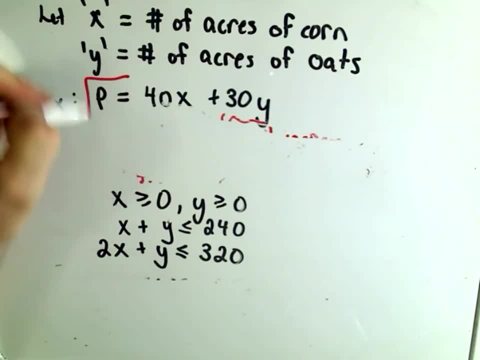 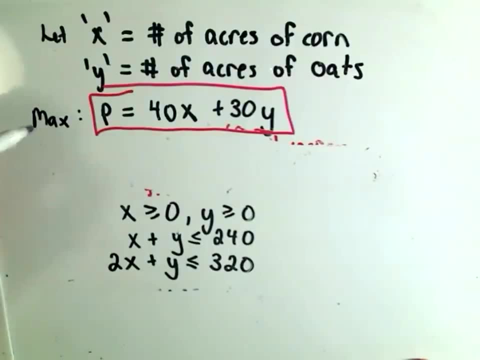 Okay, so this is what we're trying to maximize. Again, our profit equals 40x plus 30y. And now let me move these over to the side. So x has to be greater than or equal to 0.. y has to be greater than or equal to 0.. 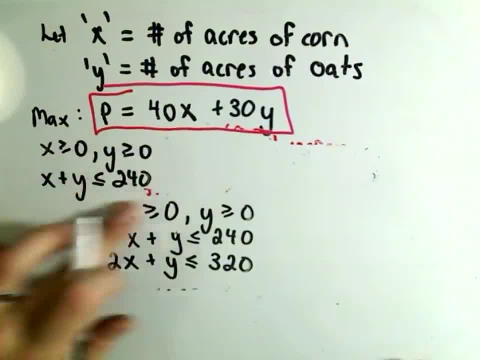 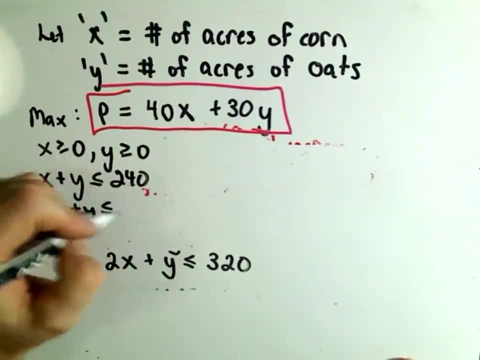 x plus y has to be less than, or equal to 240.. And then we have our other inequality: 2x plus y has to be less than, or equal to, 320.. So now all we're going to do is graph these regions. 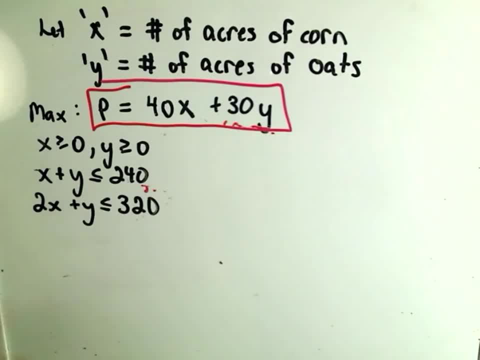 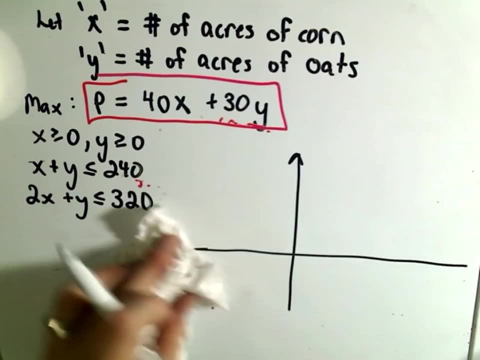 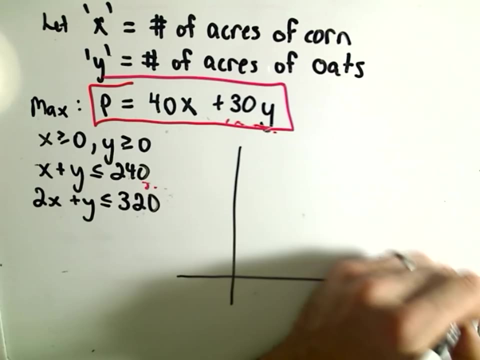 find the points of intersection and basically plug them back into our profit equation. Okay, so, Actually, let me. I'm going to redo this graph slightly. We really don't even need anything except for the top right quadrant. So there's that. 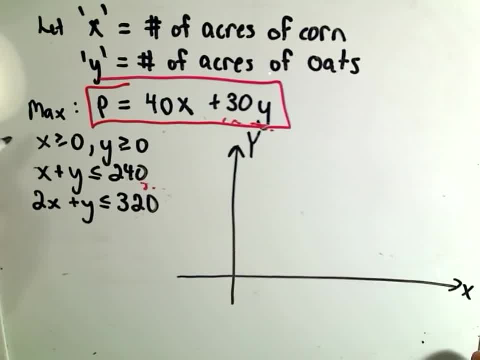 There's x and there's y. right, Because if x has to be greater than or equal to 0 and y has to be greater than or equal to 0, that only happens in the top right quadrant. If we graph the inequality, I'm going to write it. 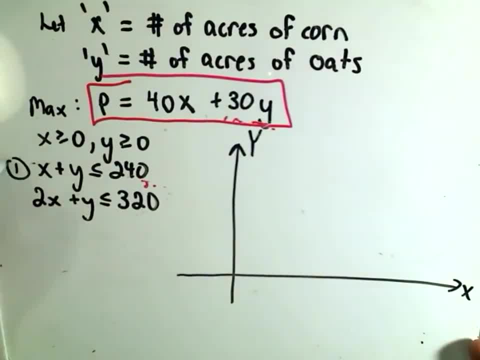 Well, you could almost think the x and y intercepts of this first inequality. If you plug in x equals 0, we'll get y equals 240.. If we let y equal 0, we'll get x equals 240.. Since it's less than or equal to, 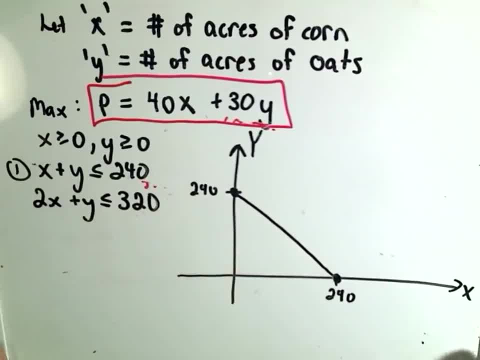 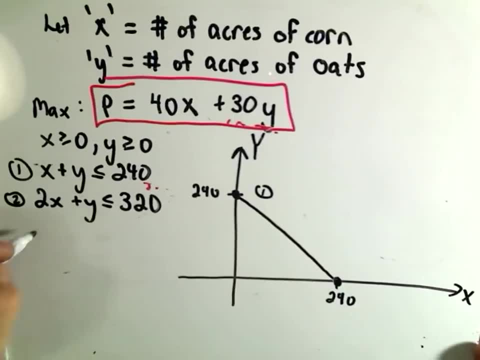 we'll make it a solid line. Likewise we could graph: So this will be the first region. Likewise we could graph the second region by finding x and y intercepts. So if we let x equal 0, if we turn this into an equation, 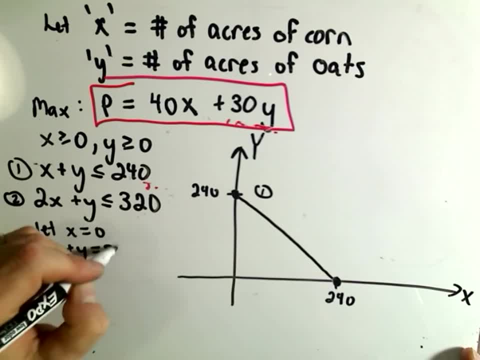 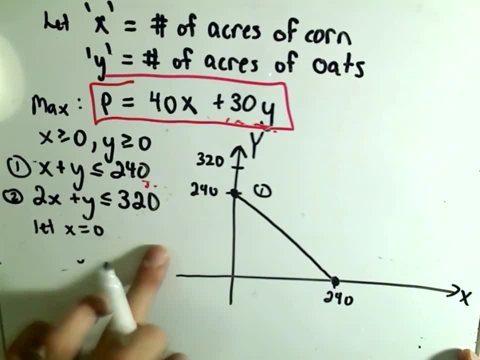 we would get 2 times 0 plus y equals 320, or, equivalently, just y is 320, so we'll make that a little higher. And then, if we let y equals 0,, we'll get 2x equals 320. 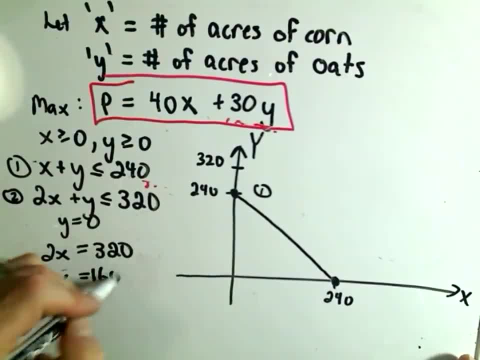 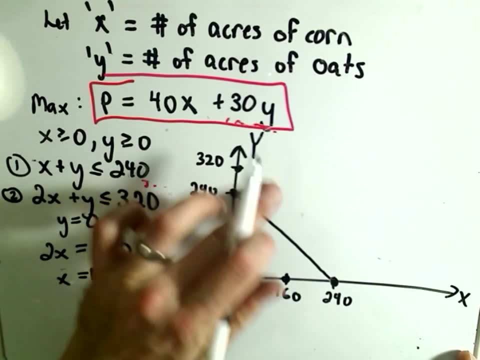 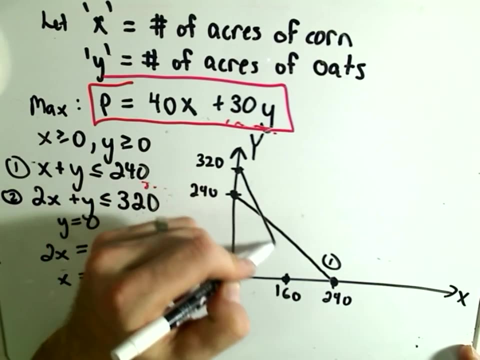 Divide both sides by 2, and we'll get x equals 160.. Okay, so not quite to scale, So we'll graph. Okay, so this is the first line over here. When we graph the second inequality, it would look something like this: 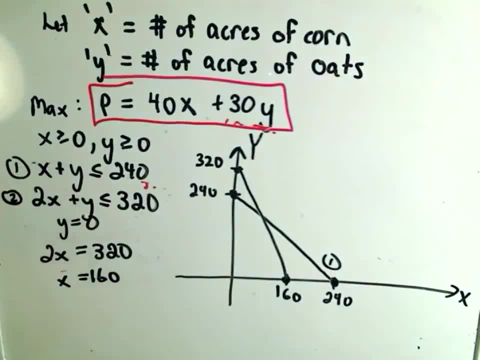 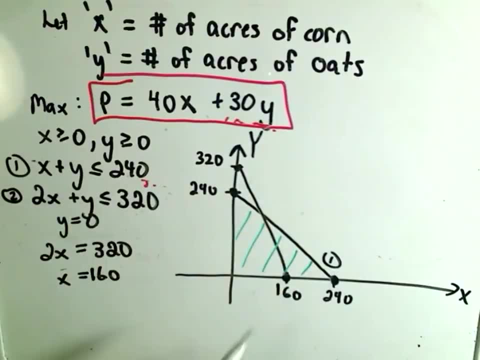 And the region that satisfies both of these inequalities is going to be the area underneath. So one part would say: okay, that would be the area or the inequality, the region we would shade underneath the first line. If we look at the second line, 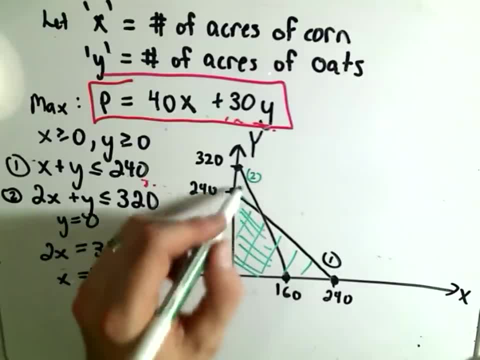 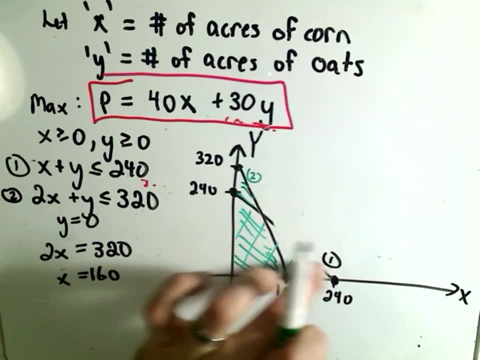 the region underneath would be that part, And we're looking basically for the overlap. so we're just going to keep the stuff in between. So I'm even going to get rid of the other lines. Okay, so now we have our little region here. 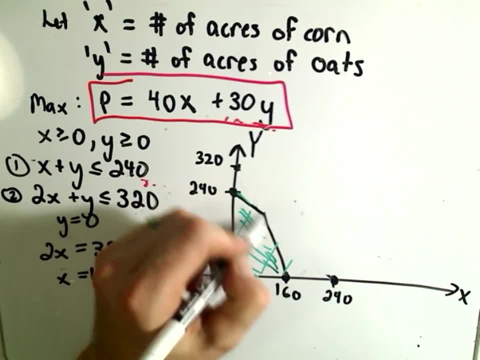 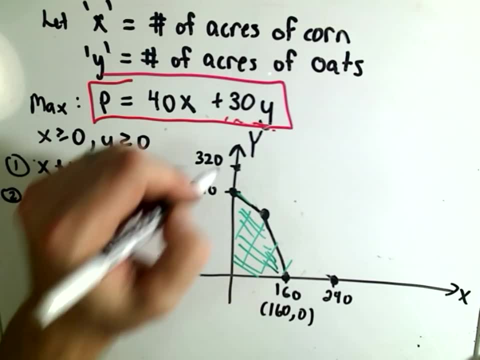 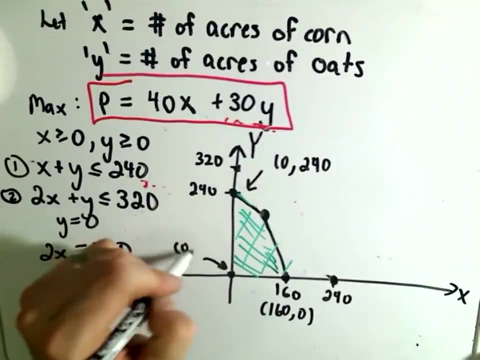 All we have to do is basically figure out the corner points, which really we already have done for the most part. We know that this is going to be the point. We know that the point up here is simply We've got the origin, which is just 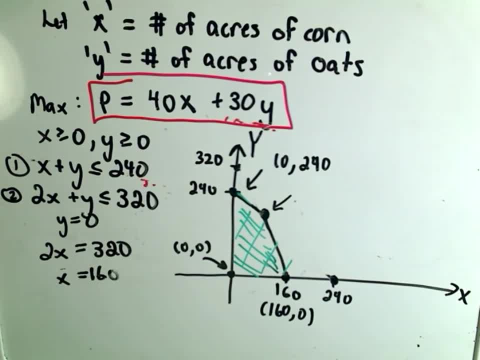 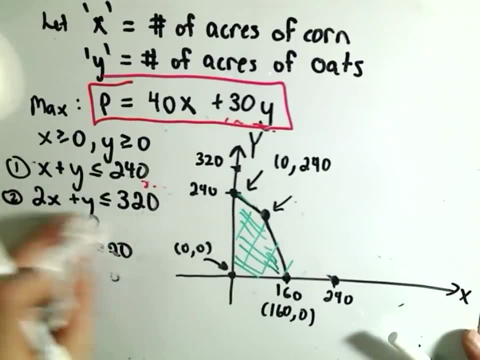 So the last thing we would have to do is figure out this other point. And if we set the lines equal to each other? so I'm going to solve for x and y here. I'm basically going to turn my inequalities into equations. So x plus y equals 240. 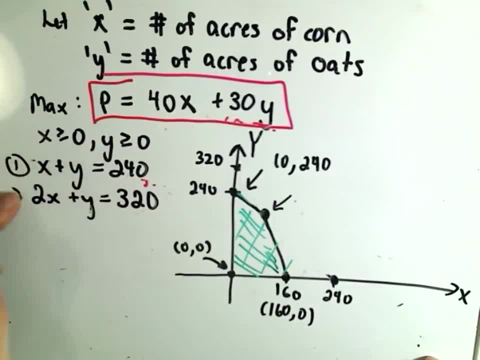 2x plus y equals 320. And what I'm going to do is I'm going to actually rewrite the first one underneath, So x plus y equals 240. And I'm going to use elimination by addition here to solve my system of inequalities. 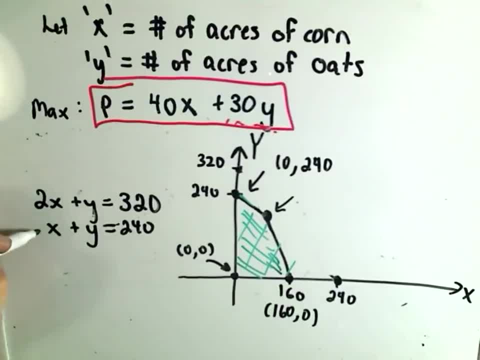 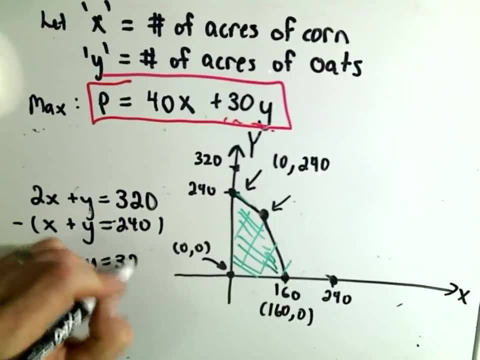 or, excuse me, my system of equations now. So multiply both sides of the first or, excuse me, the second one By negative 1, we'll get 2x plus y equals 320.. And the denominator: you'll get negative x. 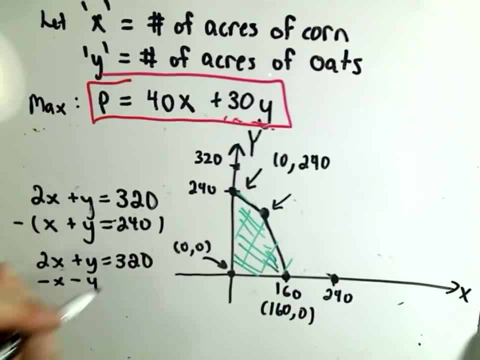 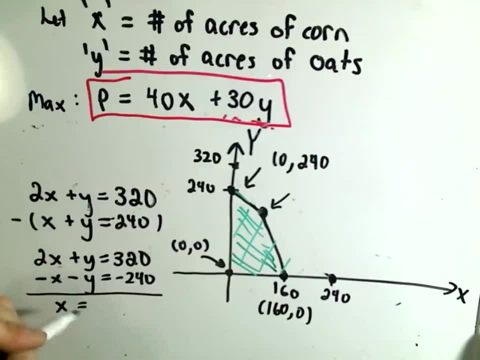 or not the denominator. but the second equation: Negative x minus y equals negative 240.. If we add these up, the x's will get 1x, the y's will cancel. 320 minus 240 is x equals 80.. 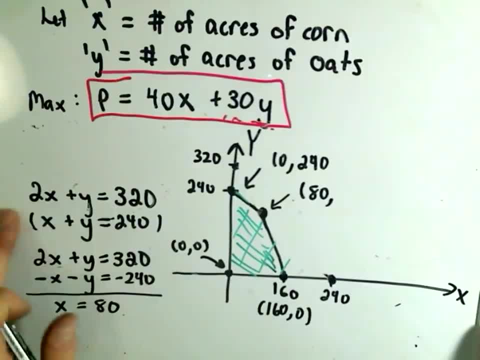 And once we know that x equals 80, we can plug that into either one of our equations to figure out the y value. So if we plug it into the first one or, excuse me, the second one, we'll get 80 plus y equals 240.. 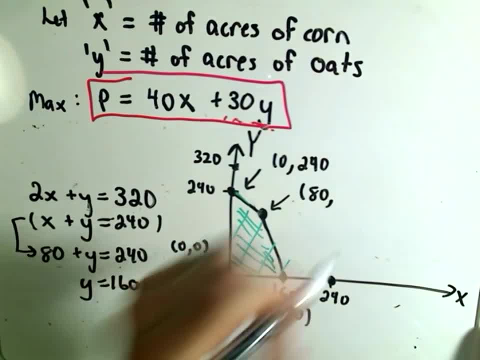 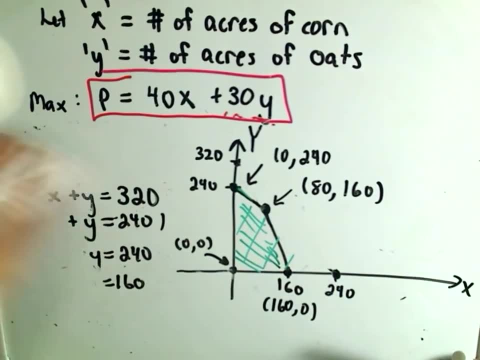 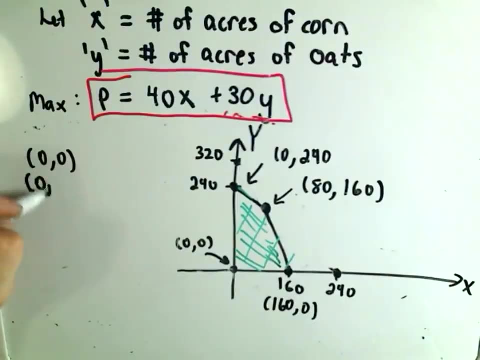 Simply subtract 80, we'll get y equals 160.. So x is 80 and y is 160.. Okay, now I have my four corner points. Okay, so we've got the points 0, 0.. 0 comma 240.. 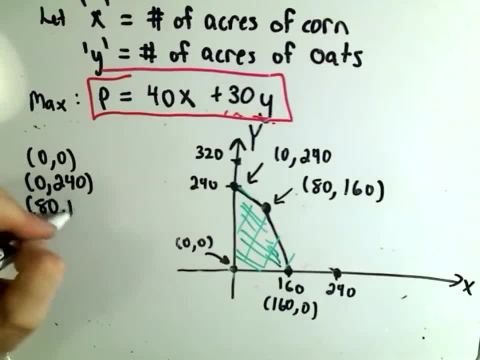 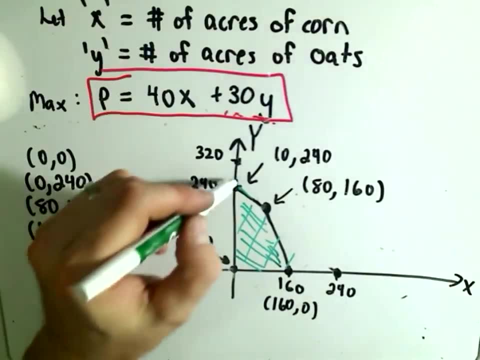 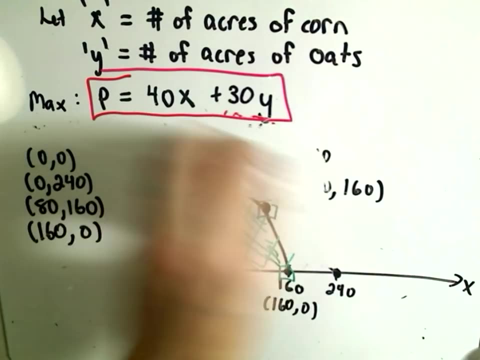 80 comma 160.. And last but not least, we have 160 comma 0.. Okay, so I'm just picking the corner points here And again. all we have to do now is just simply plug those into our function to see which is the biggest, which is the smallest. 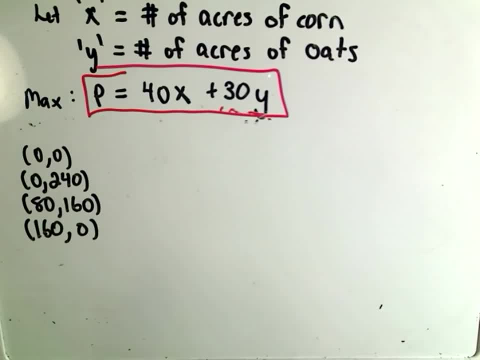 So let's see if we can't do this real quick. So certainly if you plug in 0, your profit's not going to be anything. You'll get your profit of 0, so certainly that wouldn't make sense. If we plug in 0 for x. 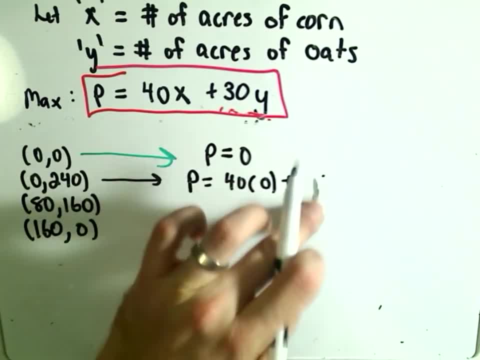 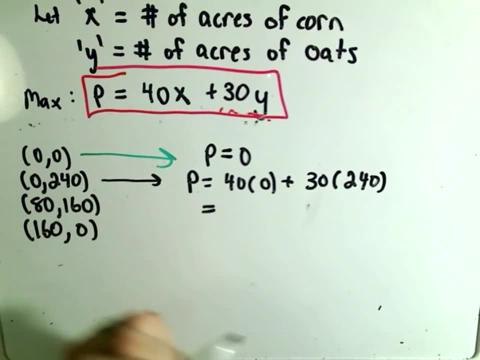 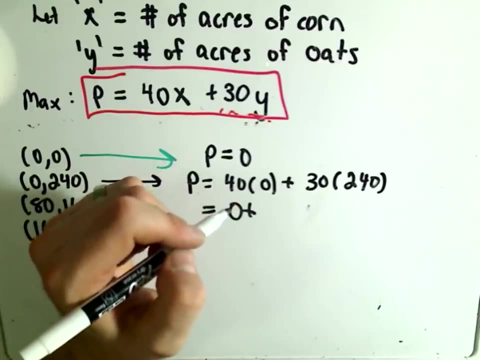 and 240, so we'll make it 240 for y. So okay, so 40 times 0 is certainly just equal to 0.. And then we'll have to add on 30 times 240.. Well, 30 times 240 is going to give us 7,200,. 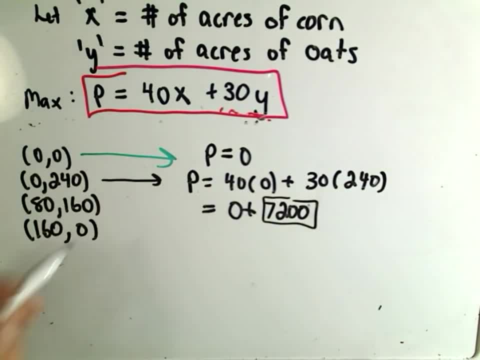 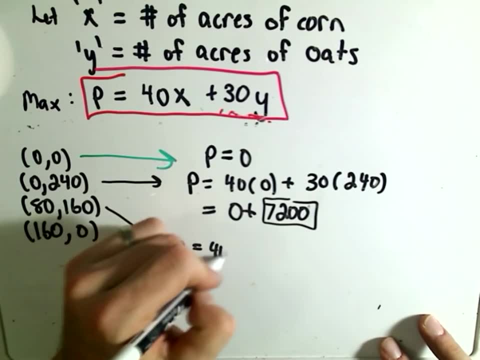 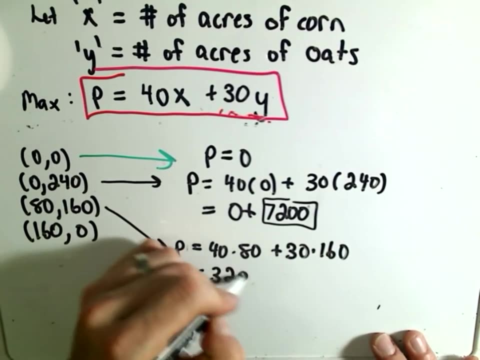 or a profit of $7,200.. Let's plug in our 80 and 160.. So our profit will equal 40 times 80 plus 30 times 160.. 40 times 80 is 3,200.. 30 times 160 is going to be 4,800. 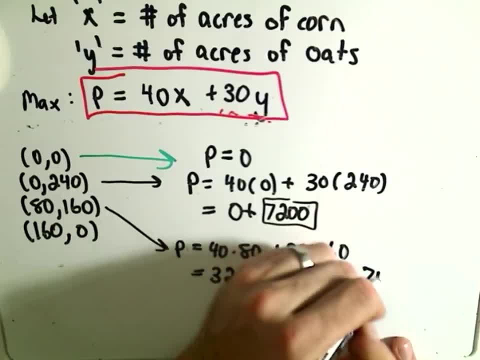 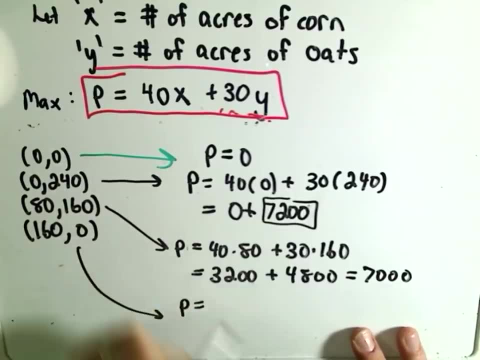 If we add these together, we get 7,000.. And, last but not least, we can plug in our 160 value. So it says our profit will be 160 times 40 plus 30 times 0, which is going to give us a profit of $6,400.. 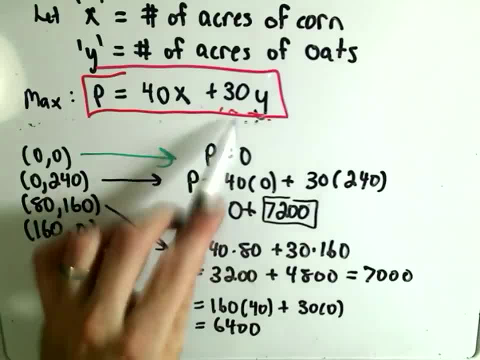 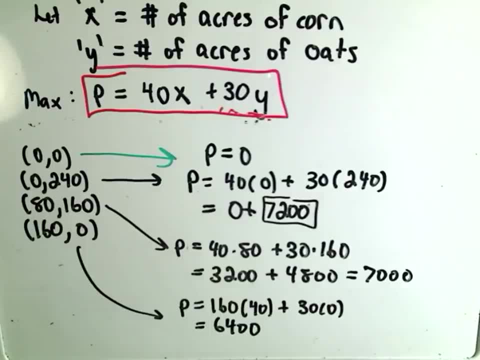 So it looks like in this case, it was actually certainly the smart thing to do. Kind of what we said was to plant all the oats, because, well, you can basically for every acre of oats, even though there's the time constraint. 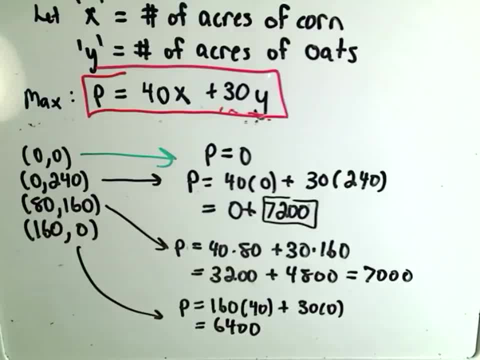 you'll actually make twice as much money. So, in this problem, our maximum, the farmer- if you're the farmer in this case- should plant all oats and you'll make as much money as possible.